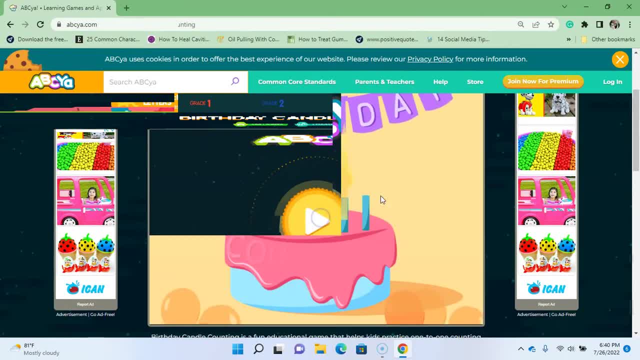 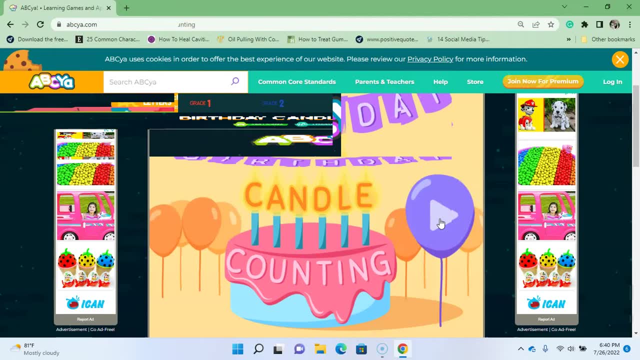 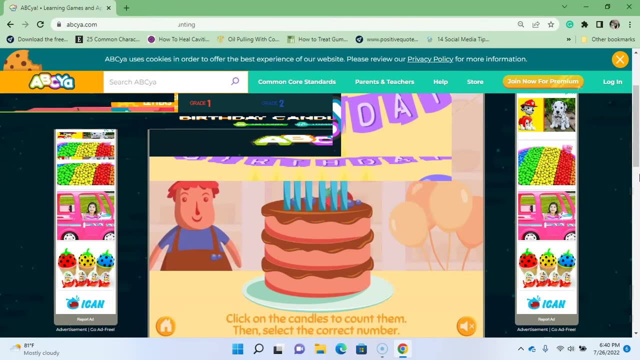 Click on that yellow play button. Let's see what we got going on Birthday candle counting. Good morning Woohoo. So click on that play button. Click on the candles to count them, Then select the correct number. How old is Dunkin' Donut? 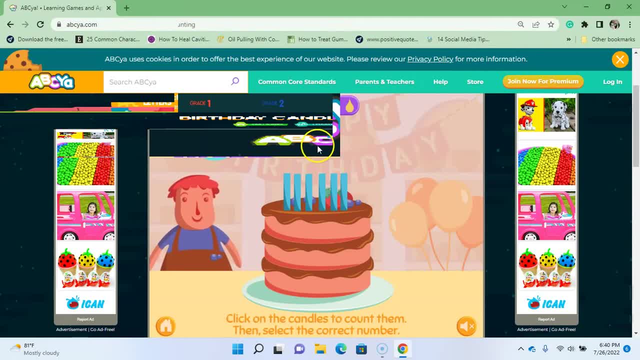 Oh, so we're gonna figure out how old Dunkin' Donut is, So we're gonna click on the candles. One, two, three, four, five, six. So we got these balloons that come up, Got two, seven, there's six. Woohoo, We got it right. 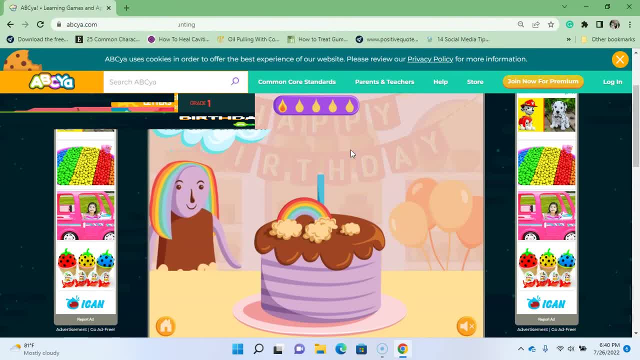 So how old is Caron Caramel? So you guys, we see these up here, We get once. we get all these, We get all these checked off. There's a kind of surprise at the end. Oh no, let's go, keep going. 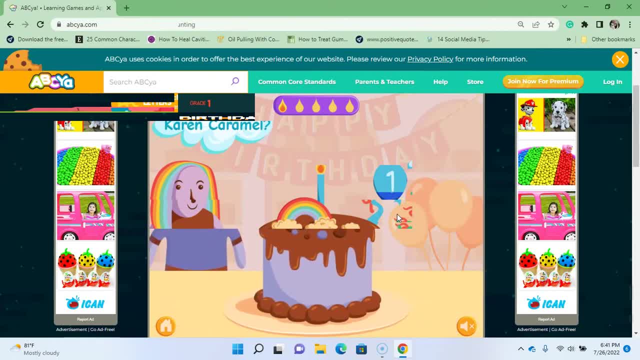 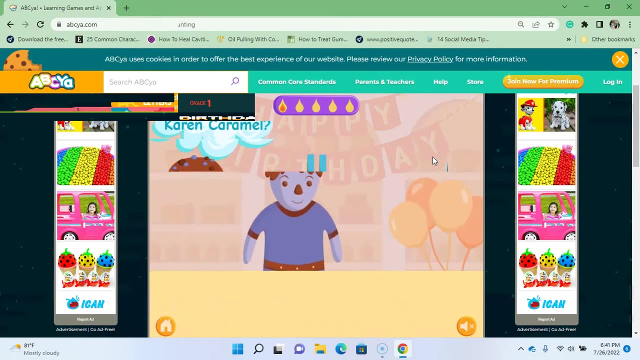 Let's see what happens at the end. Charlie Chocolate- Woohoo, Miss Lala loves chocolate. How old is Charlie Chocolate? He is two. Where's the two? There's the two. Oh, we got three going, We only need two more. 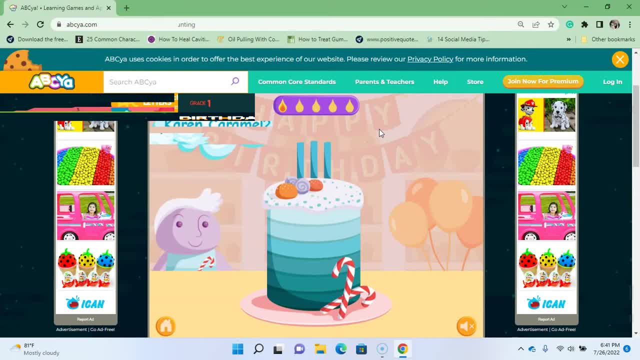 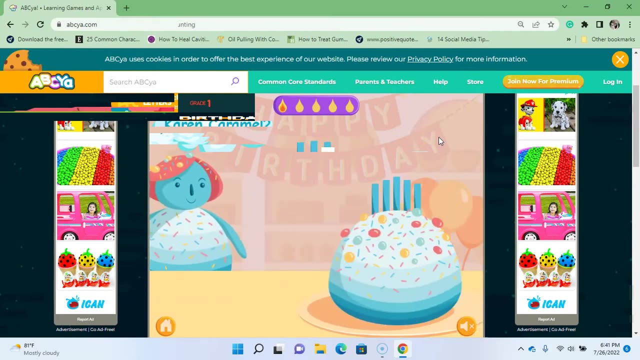 How old is Kevin Candy Cane? Oh, candy canes, Mmm. One, two, three. Kevin Candy Cane is three. Woohoo, Okay, we got one more. Let's see what happens after this. How old is Lily Lollipop? 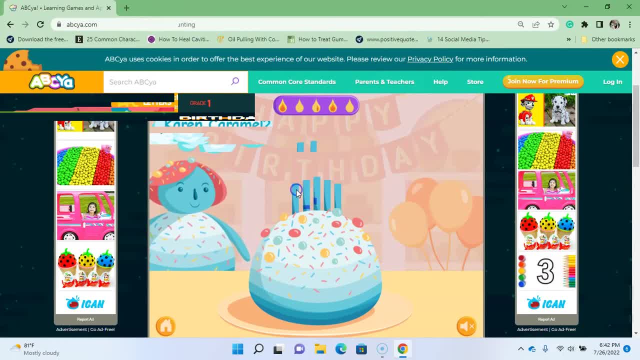 Oh my goodness. lollipops One, two, three. Lollipops one, two, three, four, five. where's the five? i see two. you guys know what number that is eight, five. oh, let's see what happens. i don't know, something's gonna happen.